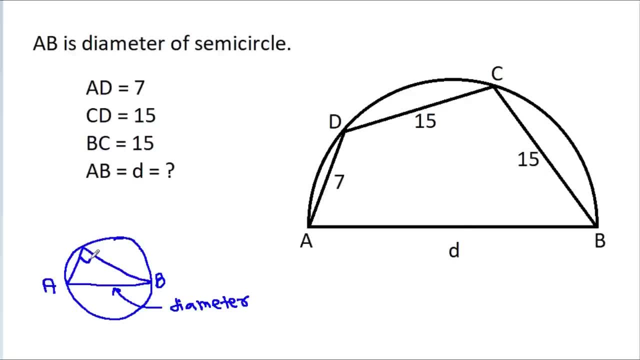 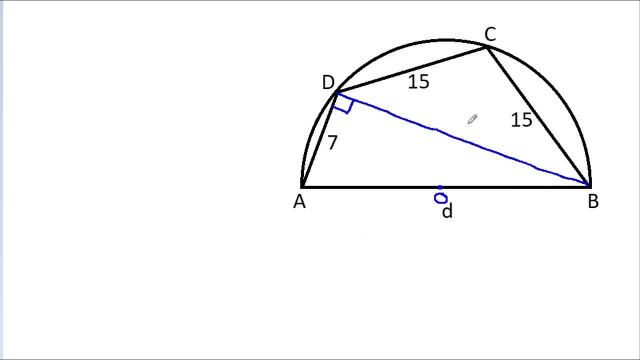 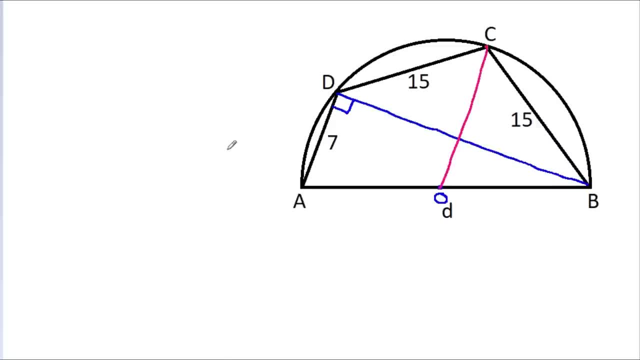 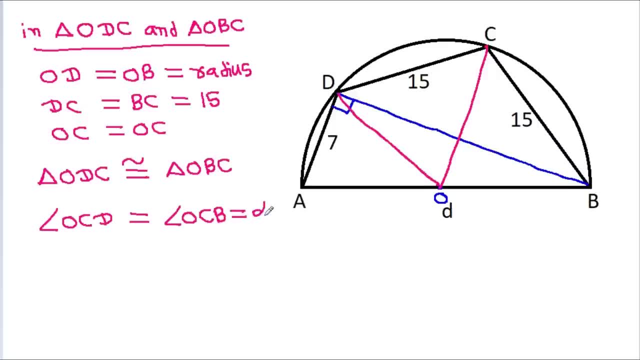 OCB. Suppose alpha: this angle is alpha and this angle is alpha Now in triangle BCD. it is BCD, CD is 15 and BC is 15. so BC is equal to CD. that means two angles will be equal. if this angle is theta, then this angle will be theta. 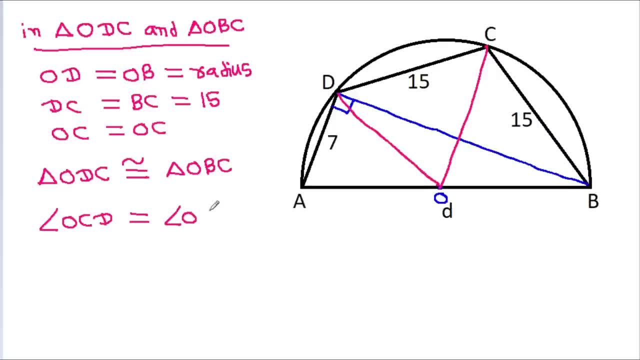 to angle OCB. Suppose alpha, this angle is alpha and this angle is alpha. And now in triangle, BCD: it is BCD, CD is 15 and BC is 15. so BC is equal to CD. that means these two angles will be equal. 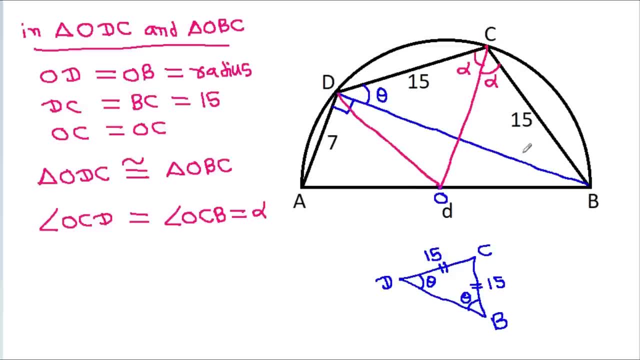 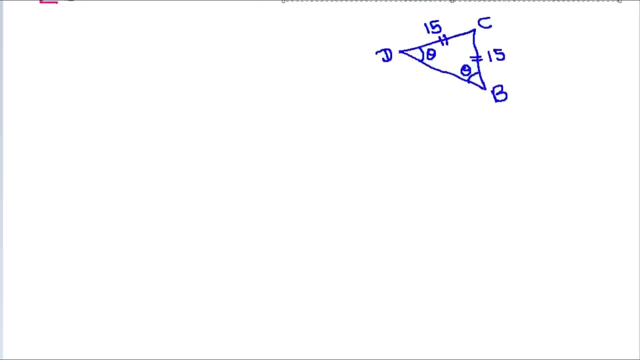 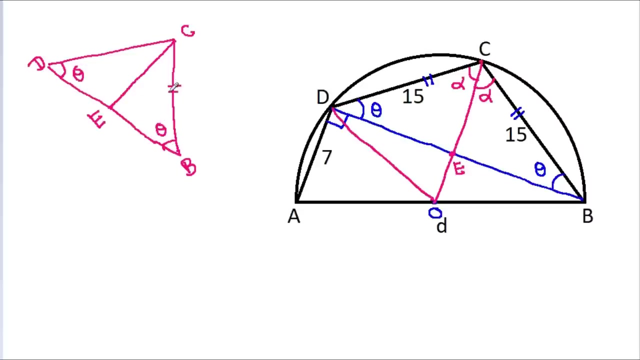 If this angle is theta, then this angle will be theta, and BC is equal to CD. and now in BCD- suppose this point is E- it is BCD and E. these two angles are equal. BC is equal to CD and these two angles are equal. So triangle DEC: it will be congruent to triangle BEC. that means DE, it will be equal to BE, and. 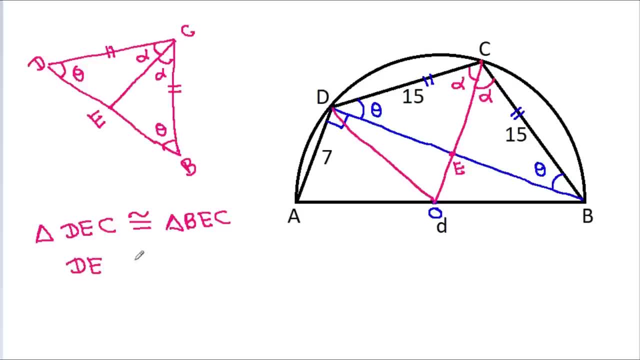 angle DEC it will be equal to angle BEC and angle DEC it will be equal to angleには DEC C, and it is B, D, E and this angle it will be 180 degree, so these two angles will be 90 degree. these angles are 90 degree, so opposite angles will be also 90 degree. 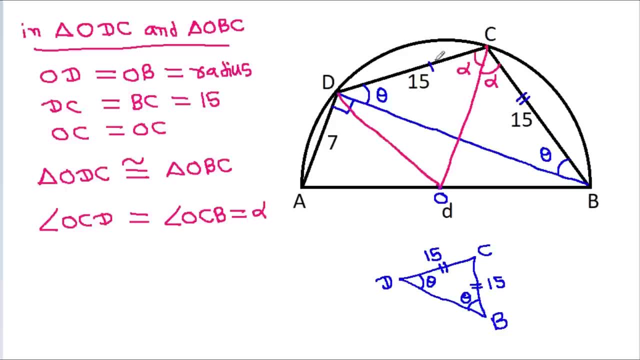 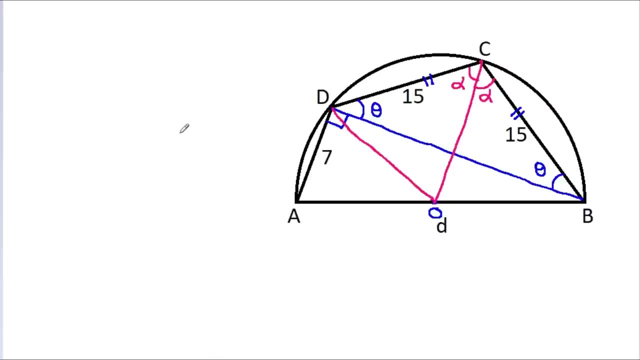 and BC is equal to CD. and now in BCD- suppose this point is A, it is BCD and E. this two are equals- is equal to B, C, CD, and this two are equal to C, D. so triangle, D is C, it will be congruent, and B is theta. 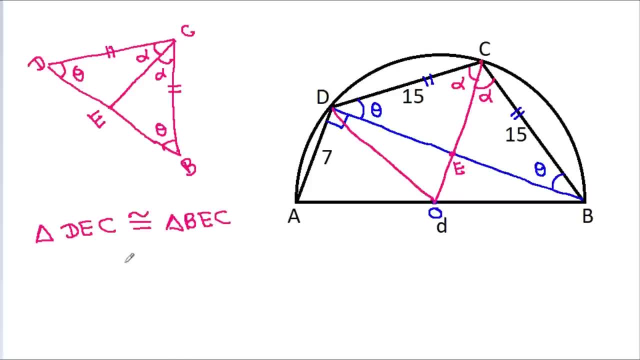 to triangle BEC. that means DE. it will be equal to BE, DE will be equal to BE and angle DEC it will be equal to angle BEC and it is BDE and this angle it will be 180 degree. so these two angles will be 90 degree. 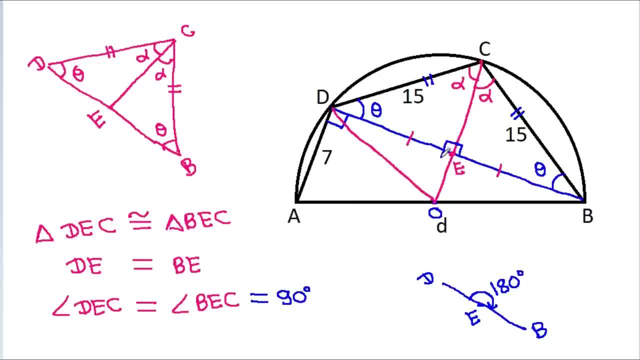 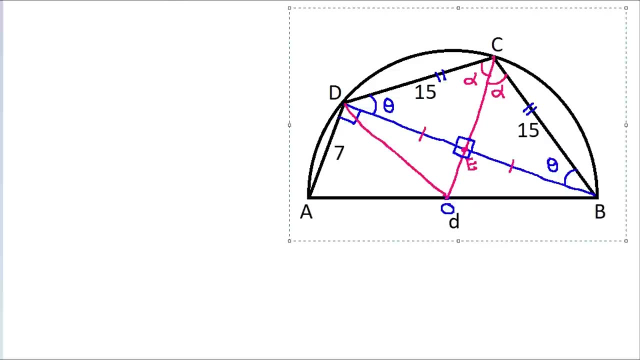 These angles are 90 degree, So opposite angles will be also 90 degree. and now in ABD, So it is ABD and OE. this angle is 90 degree. angle B is common, so in triangle BOE and triangle BAD. So 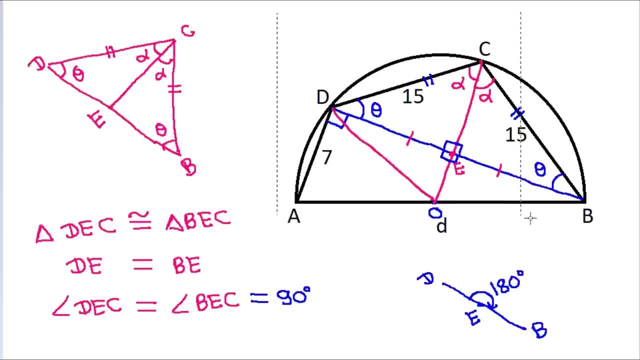 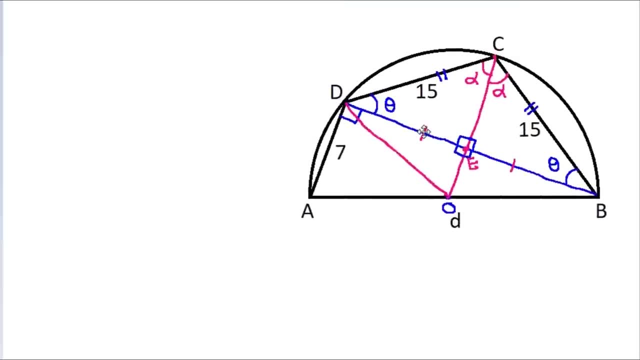 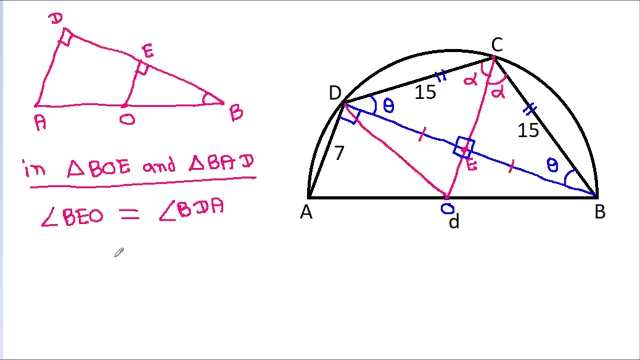 and now in ABD it is ABD and OE. this angle is 90 degree. angle B is common. so in triangle BOE angle B is common. so in triangle BOE angle B is common. so in triangle BOE and triangle BAD angle BEO it is equal to angle BDA and angle EBO it is equal to angle DBA. 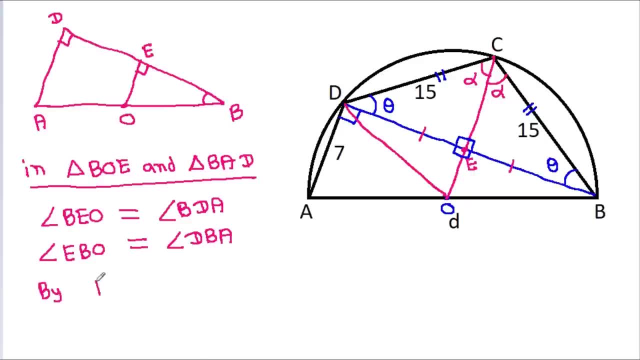 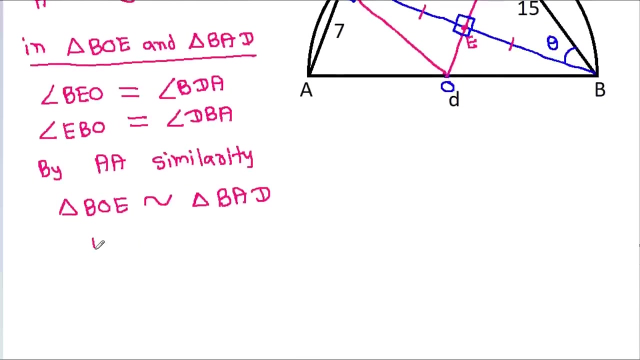 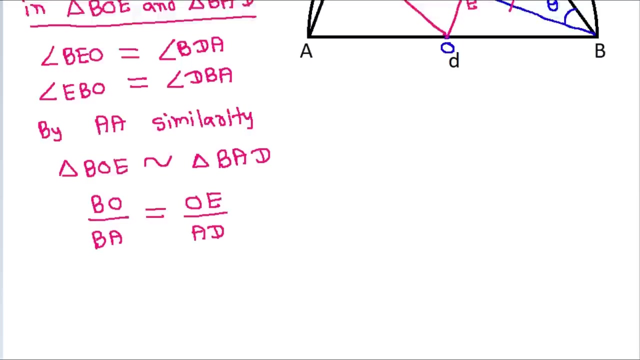 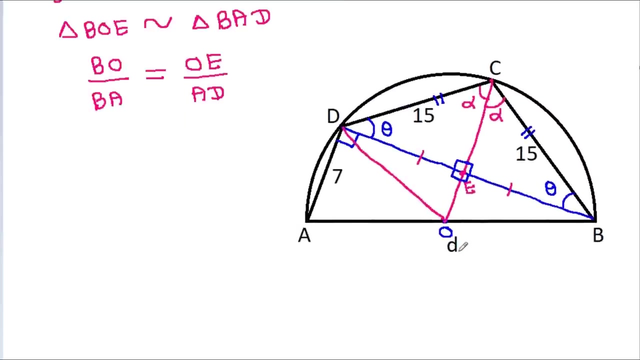 So by angle-angle similarity, triangle BOE it will be similar to triangle BAD. So BO by BA It will be equal to OE by AD. And suppose radius is R, then BO will be R, AO will be R. 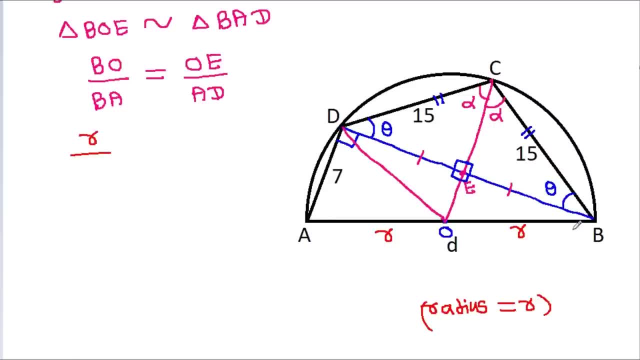 So it will be equal to OE by AD. So it will be equal to OE by AD. So BO is R and BA will be R plus R. that is equal to OE by AD is 7, and R by 2R it is equal to OE by 7, and R will get constant. 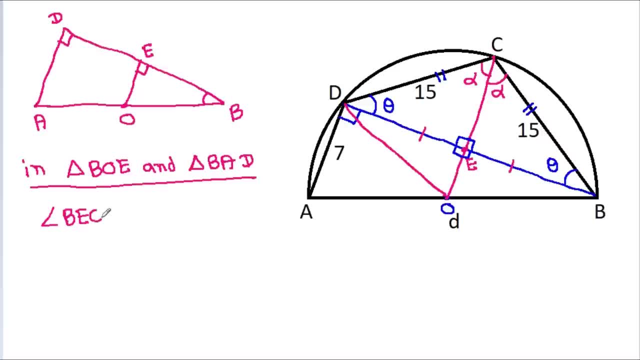 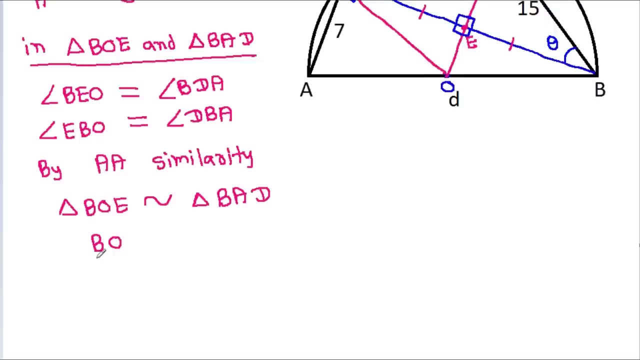 angle BEO it is equal to angle BDA and angle EBO it is equal to angle DBA. so by angle angle similarity. 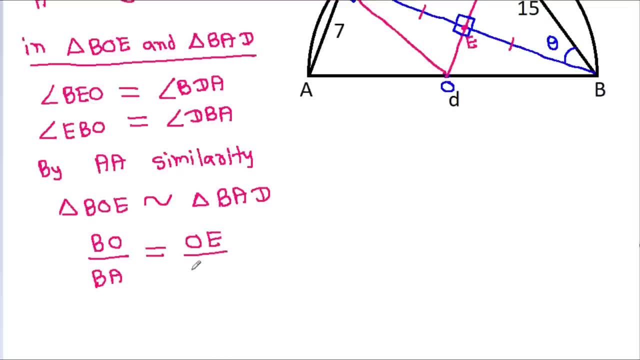 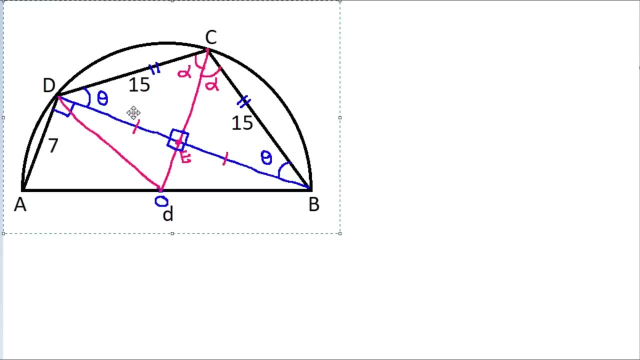 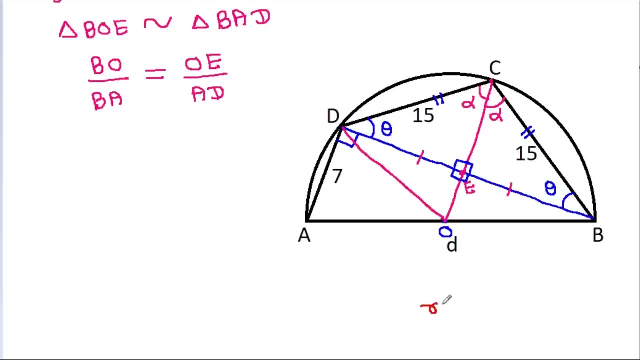 and suppose radius is r, then Bo will be r, Ao will be r, so Bo is r and Ba will be r plus r. that is equal to Oe by Ad is 7 and r by 2r. it is equal to Oe by 7 and r will. 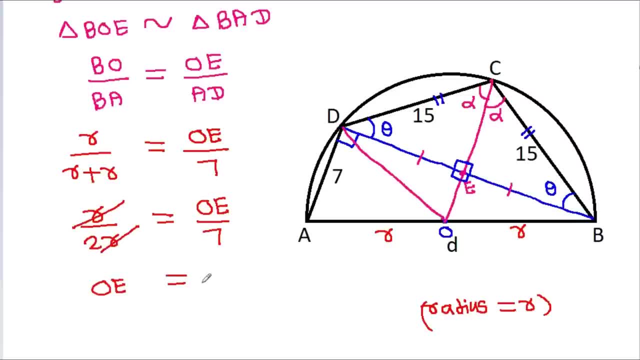 get cancelled. so Oe it is equal to 7 by 2, Oe is 7 by 2.. Ok And Oc is equal to r. that means Ec. it will be equal to r minus 7 by 2, Ec it will be. 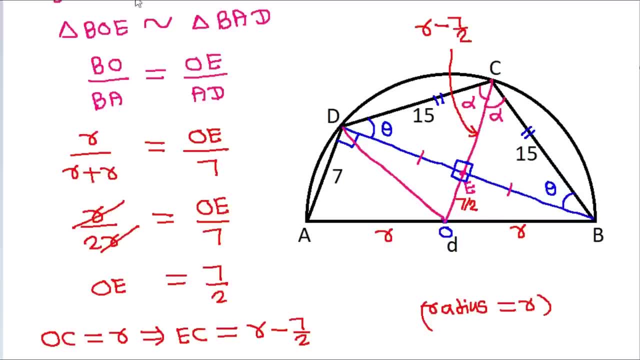 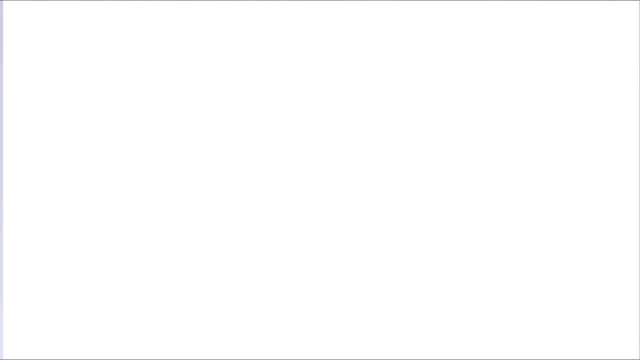 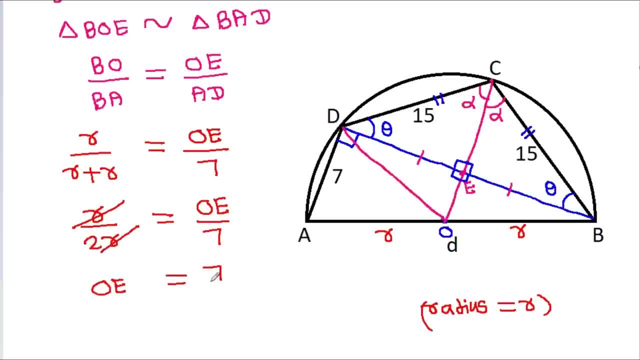 So OE it is equal to 7 by 2.. So OE is 7 by 2.. And OC is equal to R. that means EC it will be equal to R minus 7 by 2. EC: it will be R minus 7 by 2.. 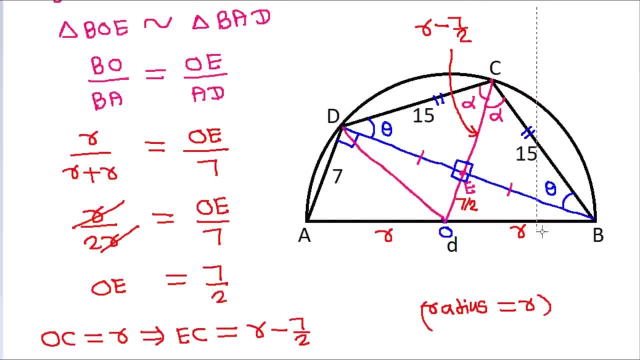 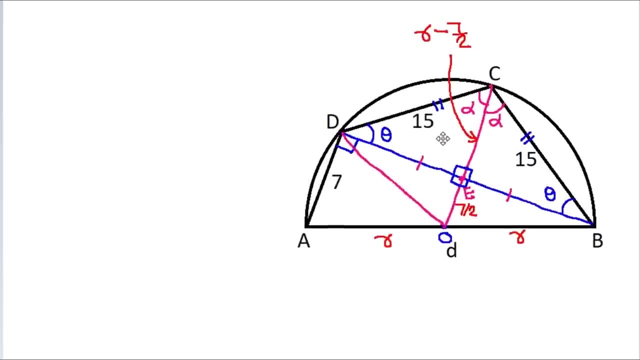 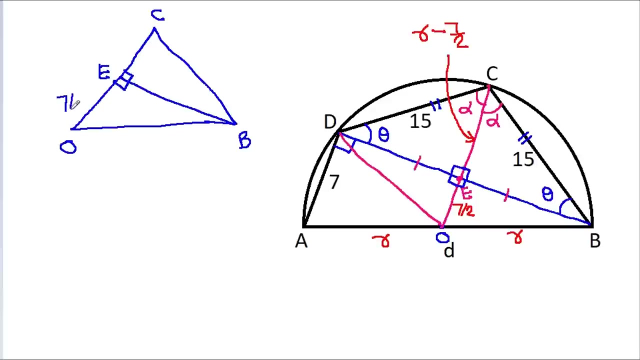 And now in OBC it is O, B, C and R And E. OE is 7 by 2. EC is R minus 7 by 2. OB is R and BC is 15. And B? E S square, it will be equal to. 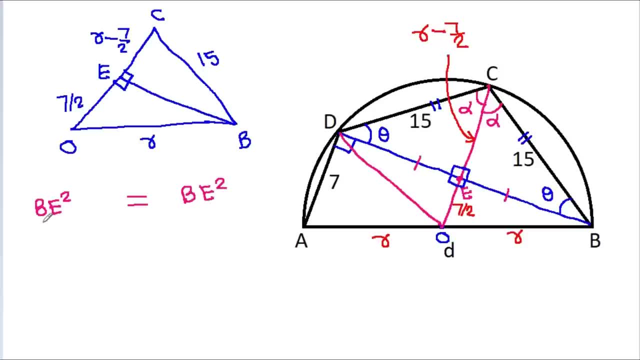 And B? E S square, it will be equal to BE S square and BE S square. it will be BO S square minus OE S square. that is equal to, And BE S square. it will be BC S square minus EC S square, and BO is R S square minus OE is 7 by 2.. 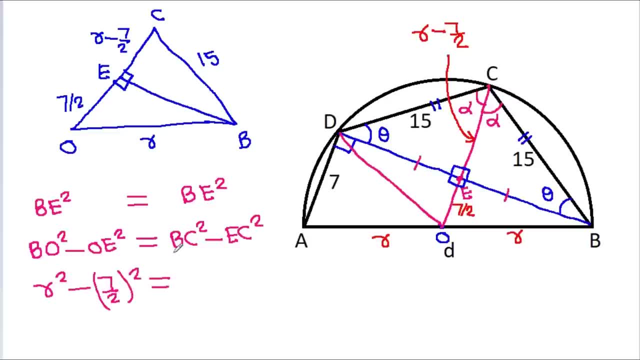 And OE is 7 by 2. S square, it is equal to BC, is 15 S square minus EC is R minus 7 by 2 S square And it is R square minus 49 by 4.. So it is equal to 225 minus R square minus 49 by 4.. 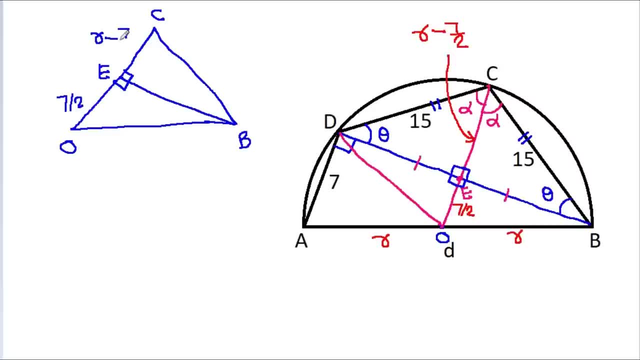 Ec is 1. R minus 7 by 2. OB is R and BC is 15 and BE square, it will be equal to BE square, and BE square. it will be: BO square minus OE square, that is equal to, and BE square it will be. 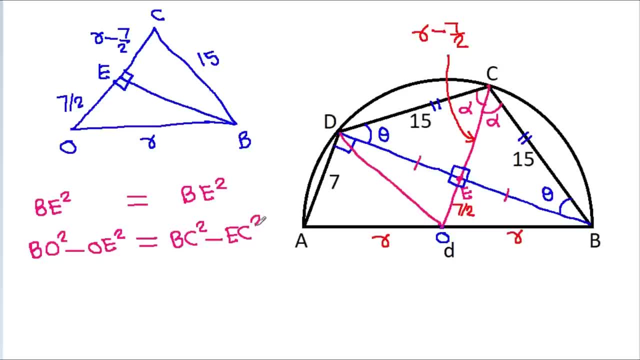 BC square minus EC square and BO is R square minus OE. is 7 by 2 square. it is equal to: is equal to: bc is 15 square minus ec is r minus 7 by 2 square and it is r square minus 49 by 4. it is equal to 225 minus r square minus 49 by 4 minus 2 times r times 7 by 2 will be 7r. 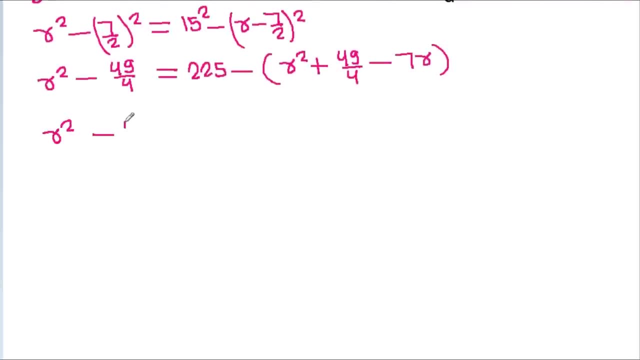 and it is r square minus 49 by 4, and it is r square minus 49 by 4 minus 2 times r. times 7 by 2 will be: 7r is equal to 225 minus r square minus 49 by 4. minus 7r and minus 49 by 4, it will get cancelled. 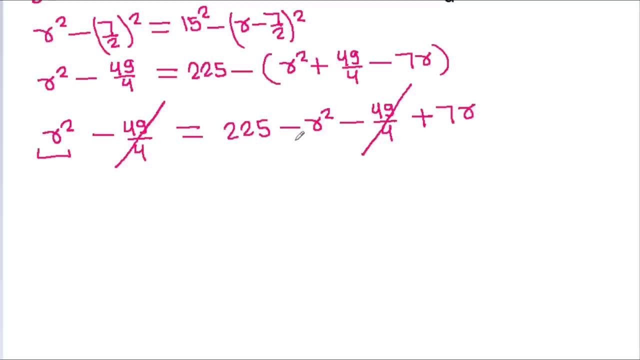 and r square minus r square, it will be 2r square minus 7r minus 225, it is equal to 0. and now we need to write: minus 7r is ar minus br, such that a minus b it should be equal to minus 7, and a times b it should be equal to 2 times 225. 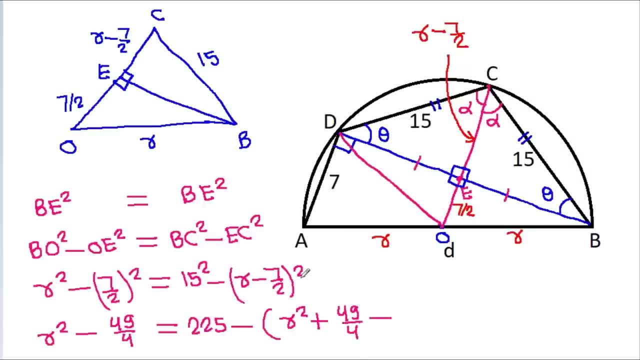 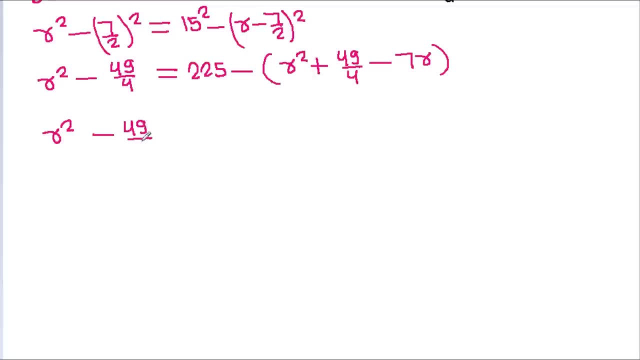 And it is R square minus 49 by 4.. So it is R square minus 49 by 4 minus 2 times R times 7 by 2, will be 7R, And it is R square minus 49 by 4 is equal to 225 minus R square minus 49 by 4 plus 7R. 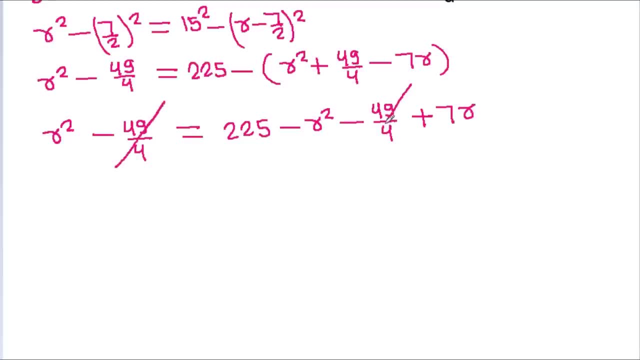 and minus 49 by 4, it will get cancelled, And r square minus r square, it will be 2r square minus 7r minus 225, it is equal to 0.. And now we need to write: minus 7r is ar minus br. 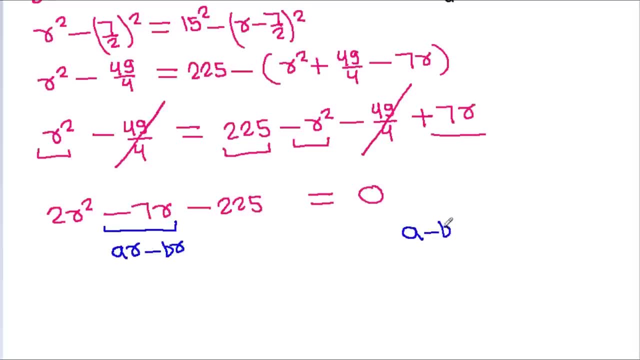 such that a minus b, it should be equal to minus seven, and a times b, it should be equal to 2 times 225, A times b is 0,, it is 2 times 225, is 5 times 45, and it is 2 times 5 times 45, is 5 times 9, and it is. 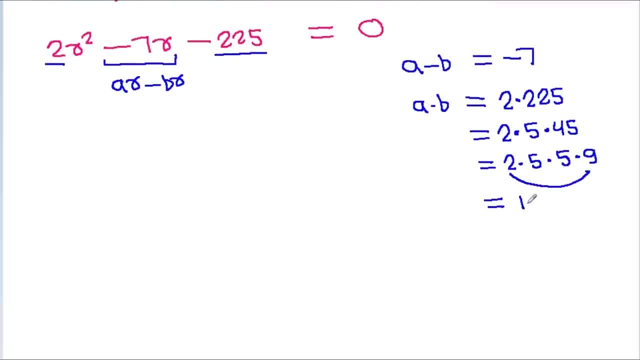 equal to 2 times 9 is 18 times 5 times 5 is 25 and minus 7 is 18 minus 25. so it is 2 R square and minus 7 R. it is plus 18 R minus 25 R. 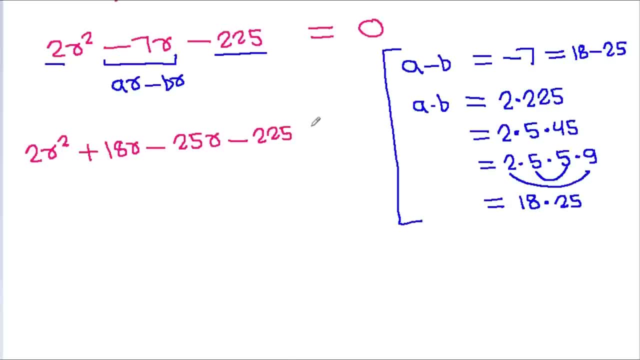 so it is 2 R square and minus 7 R, it is plus 18 R minus 25 R. so it is 2 R square and minus 7 R. minus 25 R it is equal to 0, and this is 2 R times R plus 9, and here we can take minus 25 common and it is R plus 9. that. 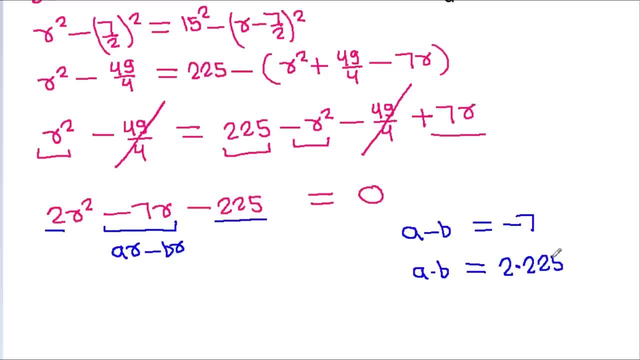 2 times 225. 2 times 225, and it is 2 times 225 is 5 times 45, and it is 2 times 5 times 45 is 5 times 9, and it is equal to 2 times 4. 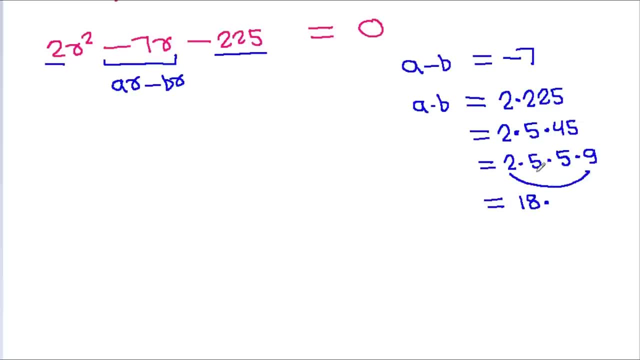 times 9 is 18 times 5 times 5 is 25 and minus 7 is 18 minus 25.. So it is 2r square and minus 7r it is plus 18r minus 25r. minus 225 it is equal to 0, and this is 2r times r plus 9, and here we can take minus 25 common. 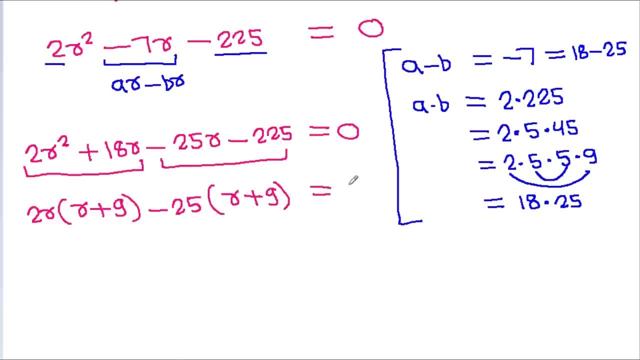 and it is r plus 9, that is equal to 0, and it is 2r minus 25 times r plus 9, it is equal to 0. so either 2r minus 25 it is equal to 0 or r plus 9 it is equal to 0. 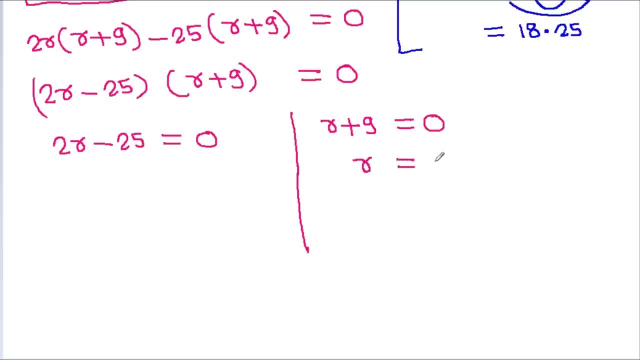 and here we get: r is equal to minus 9, but r it can not be negative, so it is not possible. and here we get: 2r is equal to 25 and diameter it is d. that will be equal to 2r, so it will be equal to 25, so d is equal to 25.. 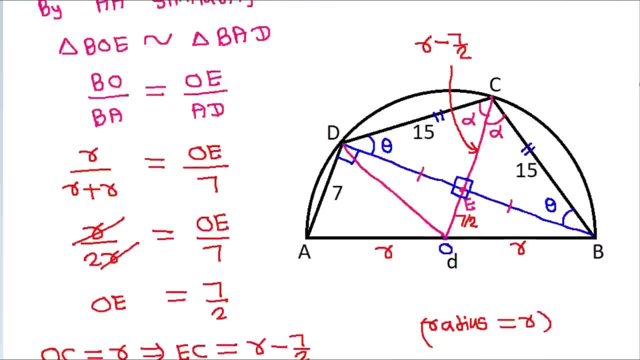 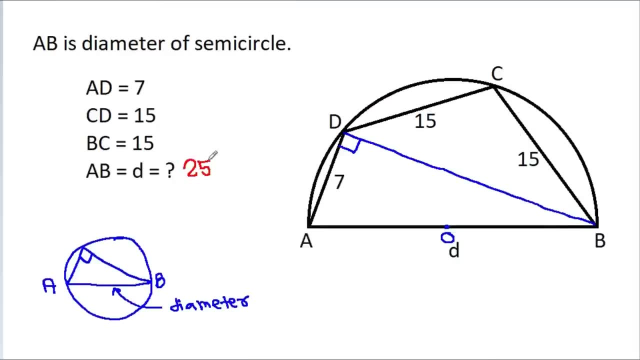 so it is 2r plus 5, r plus 9, it is equal to 25, and r is equal to 25, it is 25.. and here we get 4d, that is equal to 25, and r is equal to 4d, so it is equal to 25. and Thank you.